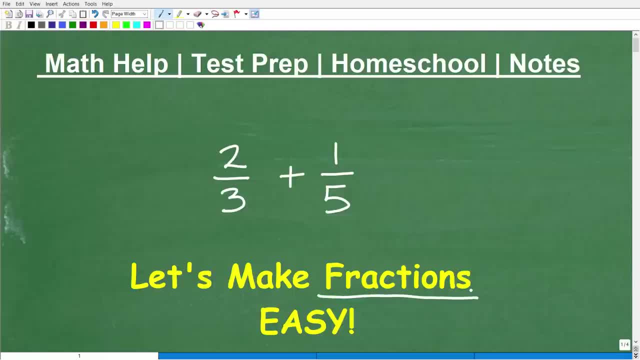 Okay, let's talk about fractions. And of course, this is everyone's favorite topic. But in actuality, most math students, when they see fractions, they have one or two expressions. Either they're very angry, they're like, fractions, just give me regular numbers like two and three. You know, I don't mind doing math when the numbers are nice and easy. But you know, some people get upset, then others are just totally just lost. They're like, oh my goodness, fractions, anything but fractions. I'll do push-ups, but not fractions. But here's the deal. If you stick with me for a couple minutes, I'm going to give you some outstanding little ways to remember how to deal with fractions. You're going to be very, very happy. And what we're going to focus on is how to do the following operations with fractions. 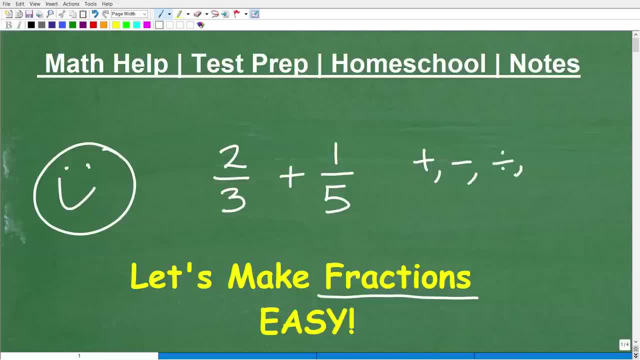 We're going to learn how to add, subtract, divide, and multiply these primary operations. Of course, most of you out there probably already learned this. 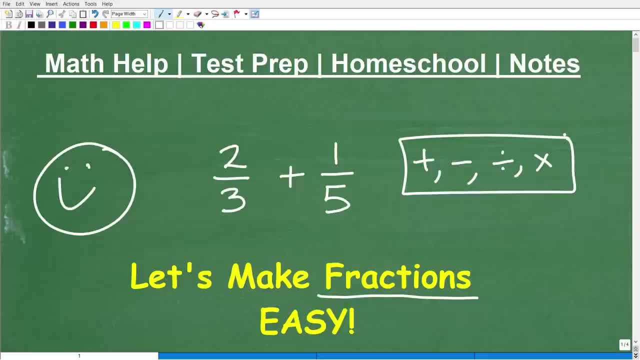 But here's the deal. Most students that have learned fractions don't really work with fractions that often, and they get confused, and they struggle because, you know, there's things involved like finding the lowest common denominator, etc., etc. But again, we're going 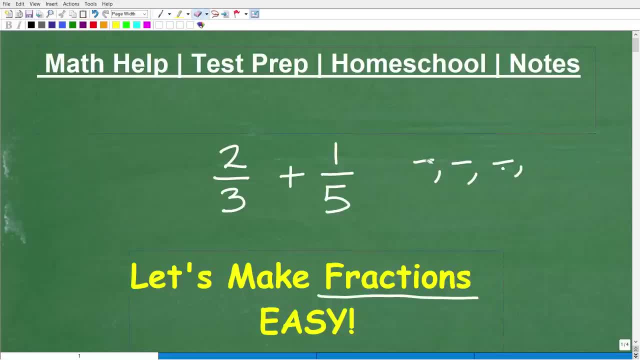 to go ahead and give you a nice quick power lesson in this video. So you're going to find fractions much easier by the time you finish this video. But I'm going to get to all of this in just 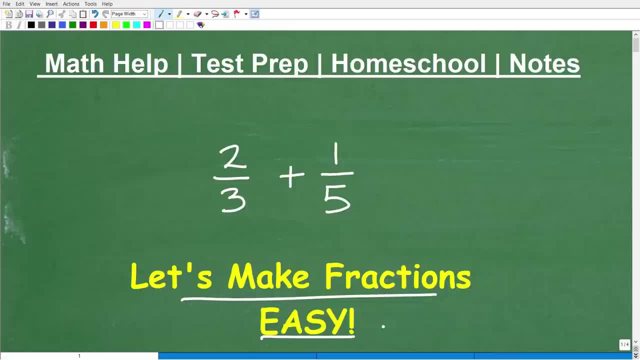 one second. But first, let me quickly introduce myself. My name is John. I'm the founder of Tablet Class Math. I'm also a middle and high school math teacher. I'm going to leave a link to all my information in the description of this video. I've been teaching math for decades, 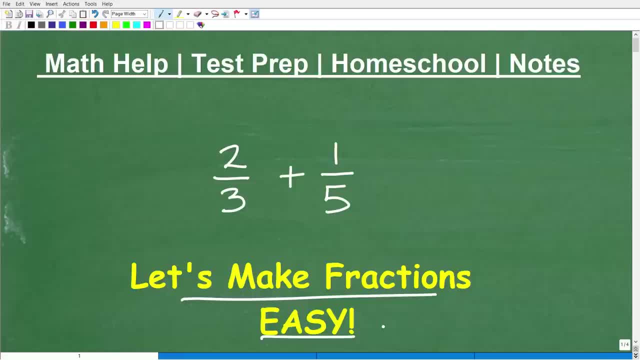 and I've come to the conclusion that all students, every single student out there can be successful in mathematics, but it requires two things. One, you have to be willing to do the work, practice, take notes, study. But that's the first thing. The second thing you need is clear and 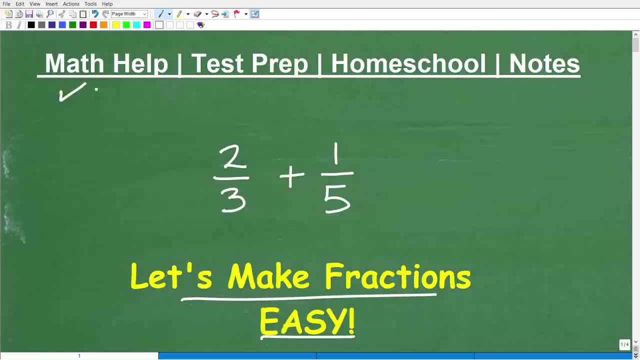 understandable instruction. So that's what I can offer you. So if you're at the middle school, high school, or even college level, you can go to the middle school, high school, or even college 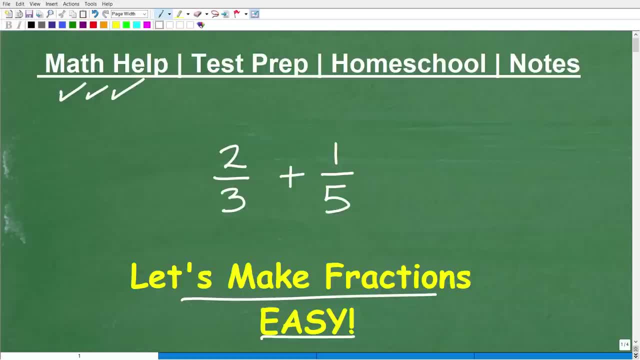 level. Definitely check out my math help program if you need assistance. By the way, if you're preparing for any test that has a math section, I'll talk about things like the SAT, ACT, maybe a teacher certification exam, GED. I can help you out there. If you homeschool, I have fantastic homeschool, middle, and high school math courses you may want to check out. And if you need some math notes, I'm going to leave links to my math notes in the description of this video as well. 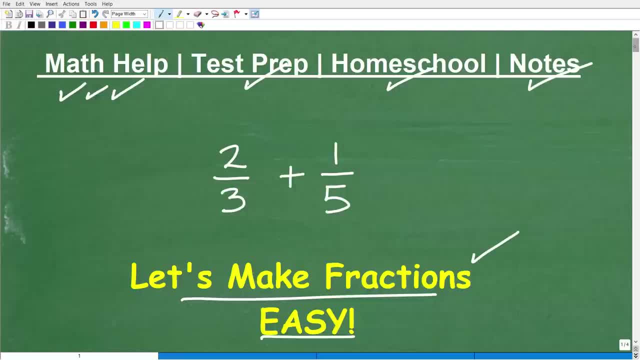 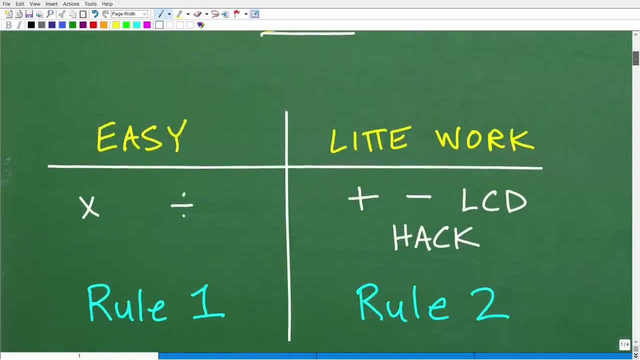 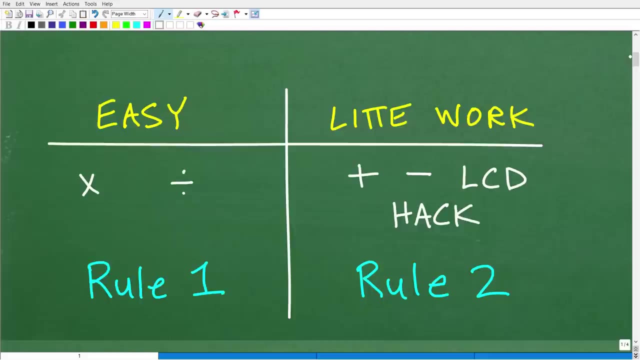 Okay, so let's get into fractions. And again, if you've been having difficulty with the fractions, that's kind of normal. A lot of students struggle with this, but we're going to make it easy for you here. So let's go ahead and first of all, set this up for us. Okay, so I want you to think of the world of fractions in kind of two rules. Okay, I'm going to break it up as one rule, and then we're going to have another rule. So the first rule, okay, is super easy. And we're talking about multiplication and division. When I show you how to multiply and divide fractions, you're going to be like, that is so easy. So we're already 50% there. Okay, so think about this four operations, we're talking about multiplication, division, and then over here, addition and subtraction. So I'm telling you right now, you're going to see how we multiply and divide fractions, you're going to be 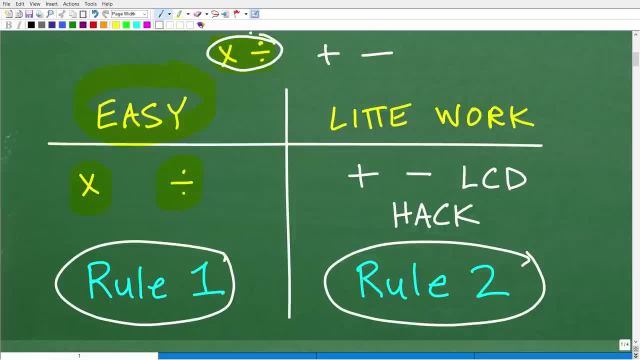 like, that is really, really easy. So that's like one rule. Okay, so that's just half of what you need to know about fractions. Now the other half is addition and subtraction. And this is where 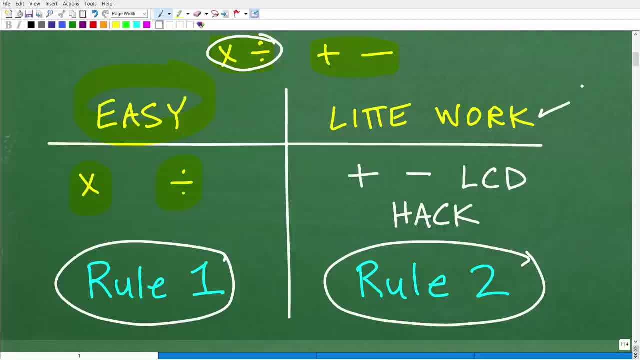 when they think of fractions, they don't like dealing with fractions, because this requires a little a little bit more work. This is when you have to do like the LCD, the lowest common denominator and all that kind of good stuff. So if you remember that, and you're like, Oh, I hate finding the LCD. Well, listen, I'm going to give you a nice little shortcut, I'm going to call it a hack that can bypass you having to find LCD. Now you still need to know how to find the LCD. 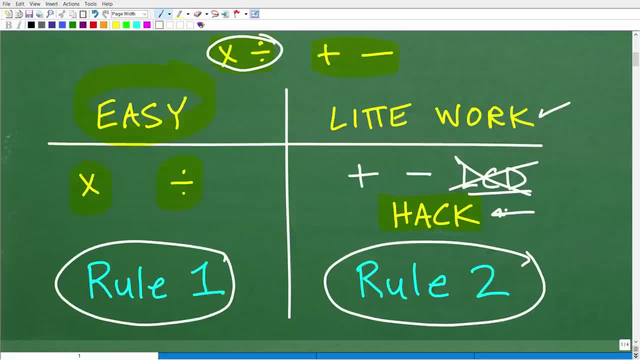 But if you're confused about this, if you'll get these problems, right, adding and subtracting problems every single time by using this nice little shortcut, you're going to want to know this for sure. And here's the great news, adding and subtracting fractions is basically the same procedure. Okay, so here's the deal. If you know how to multiply fractions, then you're 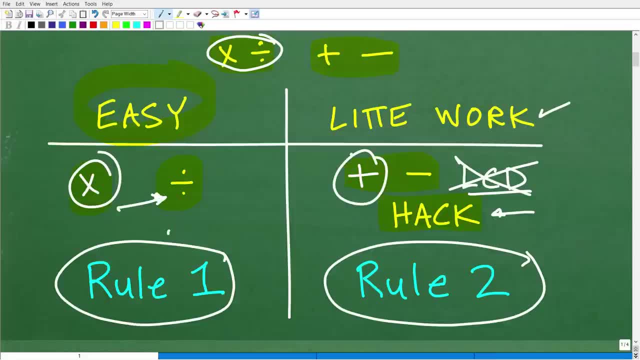 going to know how to divide, it's effectively the same thing. If you know how to add fractions, it's the same thing as subtracting. So again, just think of the world of fractions as two rules, rule one, rule two. So let's get on to this first rule, multiplying and dividing fractions 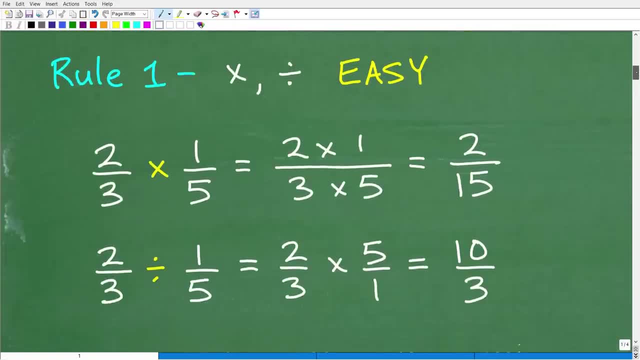 because it's super, super easy. Let's get into it right now. So our first rule, okay, multiplying 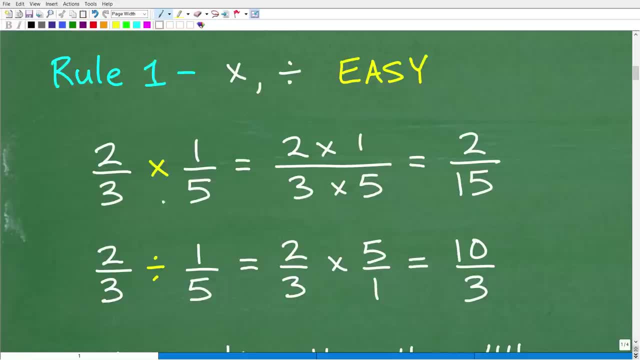 and dividing fractions, again, very easy. So let's go ahead and take a look at a couple examples. So here we have two thirds times one fifth. Now just a quick review, the top number in a fraction is called the numerator, the bottom number is called the denominator. Okay, but here's what you need to know. When we're multiplying fractions, okay, the way we multiply fractions is we simply multiply the respective numerator. So in this case, it's going to be two times one. Okay, and then we're going to multiply the respective denominators. That's three times five. I mean, it doesn't get much easier than that. So we're just going to multiply across. 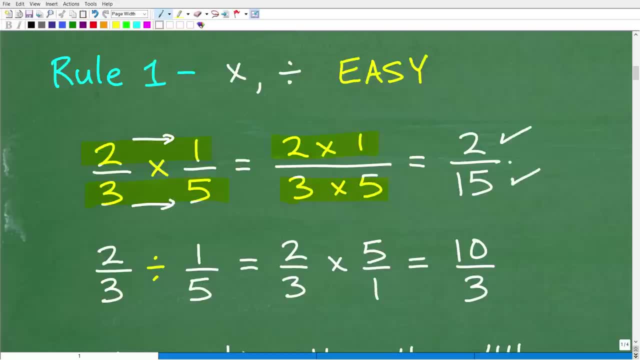 So two times one is two, three times five is 15. You are done. There is the answer. And let's go 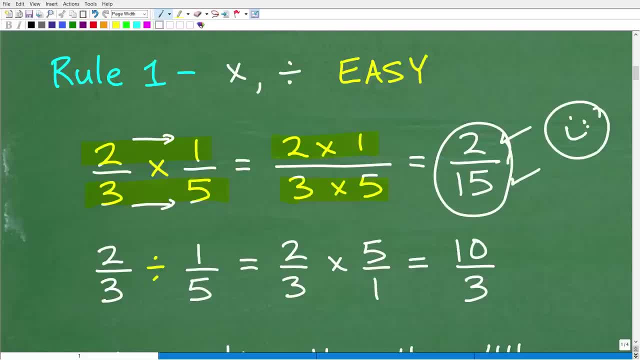 for, you know, feeling good about that. Like, hey, I know how to multiply fractions now. It's literally as easy as that. Okay, so let's talk about how to divide fractions. Now, dividing fractions, what we're going to do is take division problems, and we're going to convert them into multiplication problems. So we don't really divide fractions per se. I mean, technically, yes, that's what we're doing. But we're going to change the problem into a multiplication problem. 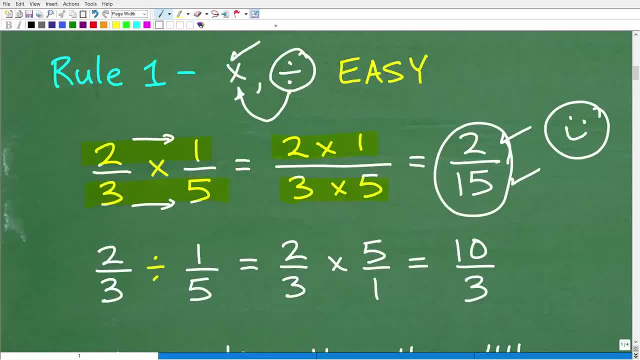 And being that you already know how to multiply, you're gonna see how easy this is so let's take a look at this problem 2 thirds divided by 1 5th okay so we're gonna change this problem from division to multiplication okay but how do we do that well you have to pay attention to the fraction to the right of the division symbol okay this division operator right there the fraction to the right of it is 1 5th okay now here's how you change this problem to multiplication you simply take the fraction to the right of the division symbol and you flip it upside down so if this is 1 over 5 we're gonna flip it upside down to 5 over 1 that's called the reciprocal okay so that's all you do and now this becomes a multiplication problem so again we're gonna go from division to multiplication by flipping the fraction to the right of the division symbol and now you already know how to multiply fractions we're gonna multiply across so that's gonna be 2 times 5 of course is 10 and 3 times 1 is 3 and we are done okay so we'll give ourselves a nice little happy 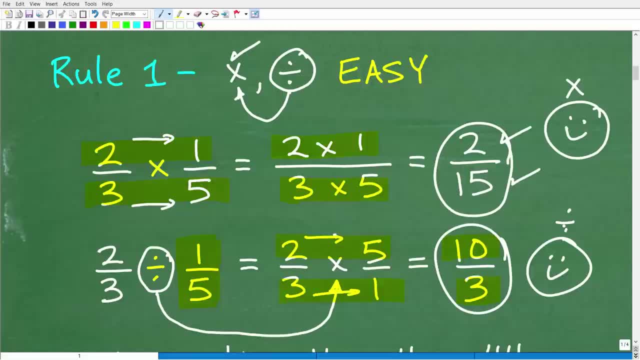 face for this so here you know how to multiply here you know how to divide now of course you're gonna want to practice this but literally this is how easy this 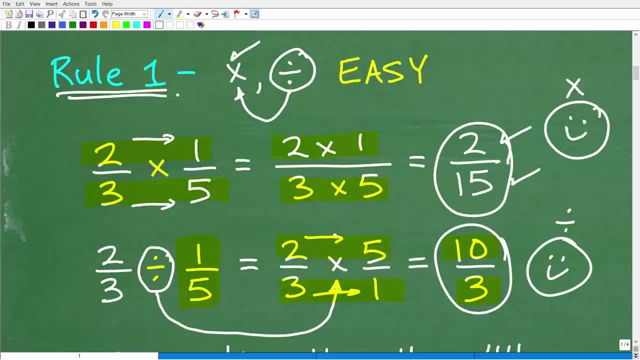 is okay so I told you this first rule rule 1 which covers multiplication and 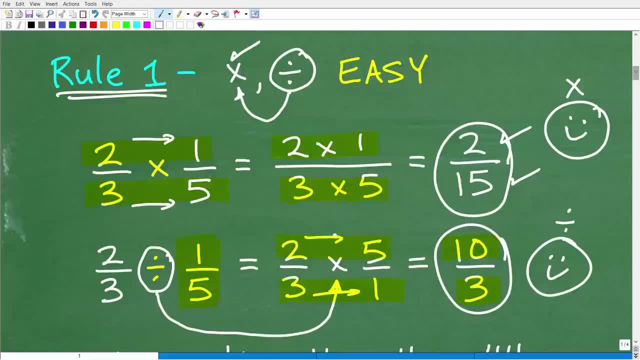 division division is very easy okay let's go ahead and add in something here okay just to make sure we're kind of complete because somebody might be thinking well what about when we're dealing with mixed 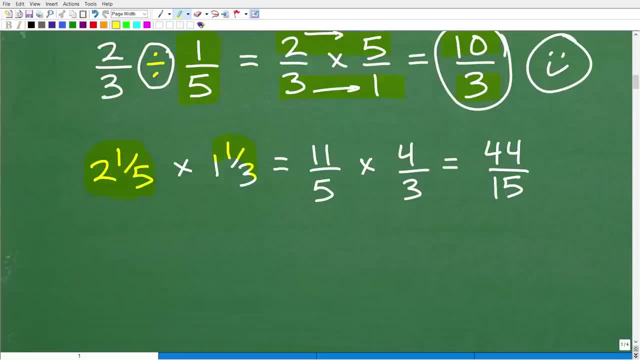 number fractions something like 2 and 1 5th and we're gonna multiply it by 1 and 1 3rd well how does that work well but you are what you're gonna want to do is rewrite these fractions as improper fractions so for example 2 and 1 5th I can write that as a single fraction by going 5 times 2 that's what that's 10 then I add 1 and 1 5th and we're done we're done so we're going to go ahead and 1. So that's going to be 10 plus 1 or 11 fifths, okay? And then 1 and 1 third as an improper fraction is 3 times 1 is 3 plus 1 is 4 or 4 thirds. So I'm going to rewrite this problem with mixed number fractions as 11 fifths times 4 thirds, okay? So now I'm just going to simply 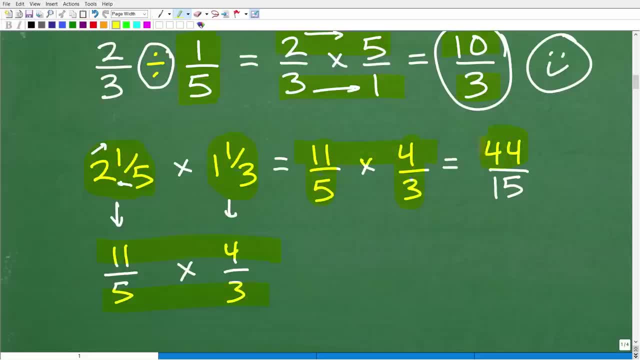 multiply across. So 11 times 4 is 44 and 5 times 3 is 15 and we are done, okay? Again, 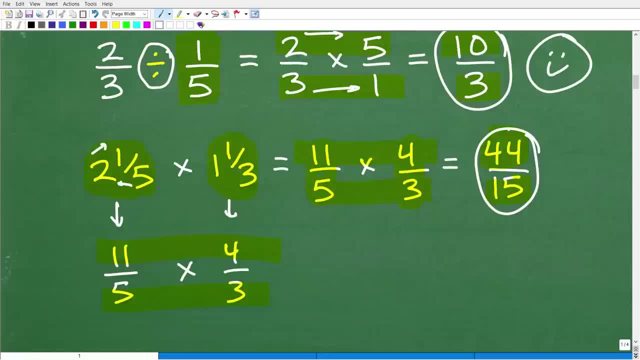 very, very easy. And now we're 50% done with learning fractions, okay? You already know how 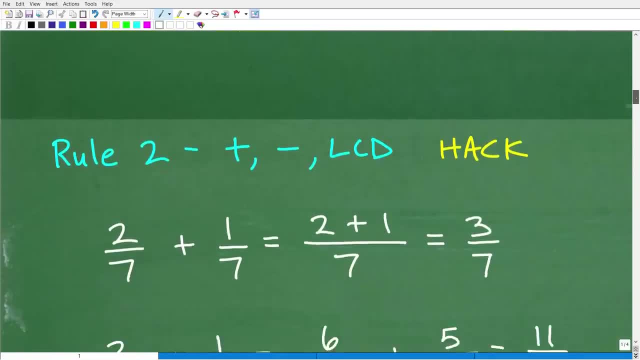 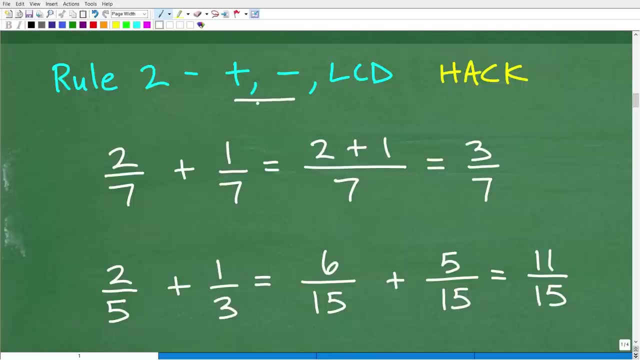 to multiply and divide. Okay, so let's get into our second rule here. And our rule number two is going to be focusing in on how to add and subtract fractions. And again, this is where you have to be thinking about the lowest common denominator. So let's get into our second rule here. And our rule number two is going to be focusing in on how to add and subtract fractions. 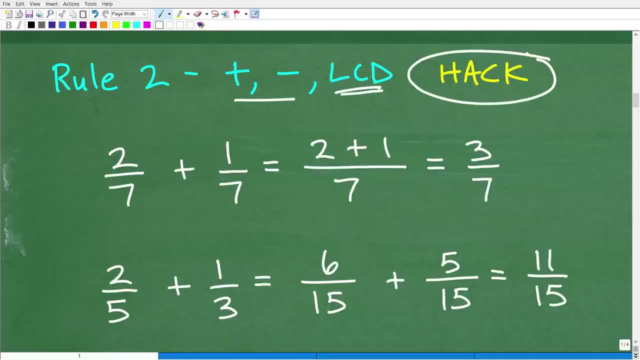 Again, this is where you have to be thinking about the lowest common denominator. But I am going to give you a lovely hack here in just one second. It's like a shortcut, okay, that you don't even have to do fraction problems using the lowest common denominator. You still need to understand it. But I'm going to give you a technique that if you're struggling with fractions, you can do addition and subtraction problems right, correct every single time. Okay, so let's go ahead and first just review some basic concepts about adding and subtracting fractions. Again, when you're adding fractions or subtracting fractions, you're doing the exact same thing. Okay, that's why I'm going to just classify this as one rule, we'll call it rule number two. All right, so here's the deal, you can add or subtract fractions, if you have the exact same denominator. Okay, the denominators must be the same. So let's take a look at this problem here, I have two sevens, plus one seven. So I'll look at the denominators. I'm like, are they the same? This is seven, that's seven. So our answer is going to have a seven as a denominator. 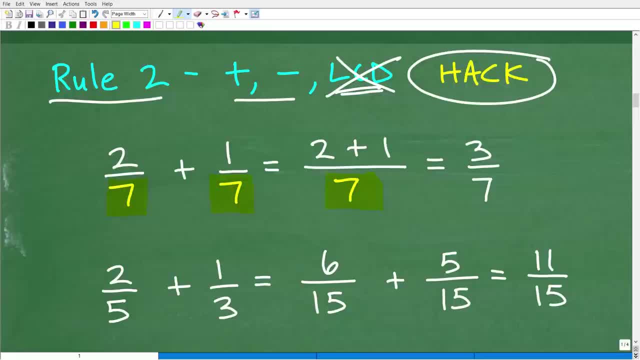 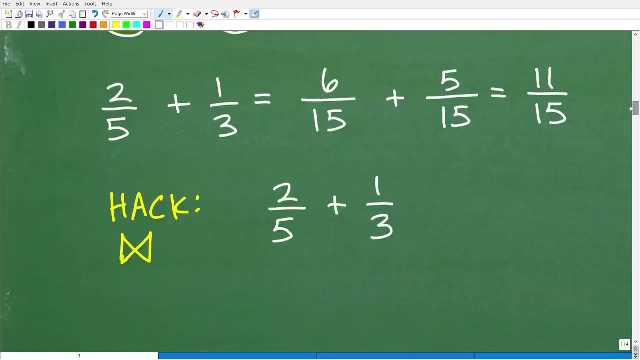 So if the denominators are the same, we're going to keep that denominator in our answer. And then we're going to add the numerators. So this is two, and this is one. So that's going to be two plus one, okay, it's going to add the respective numerators. If the denominators are the same, if this was a subtraction problem, I would subtract the numerators. But in this case, two plus one is three, and that'd be three over sevens. And that is it. Okay, so pretty easy to add and subtract fractions, especially if the denominators are the same. Okay, so if the denominators are the same, we simply add or subtract the respective numerators, and we'll get our final answer. So again, that's not that difficult. But here is where the fun starts. Okay. So what happens when the denominators are not the same? Well, this is when most people go, Oh, this is where I had to think about the LCD and everything else. That is true. Okay, you do need to think about what the LCD 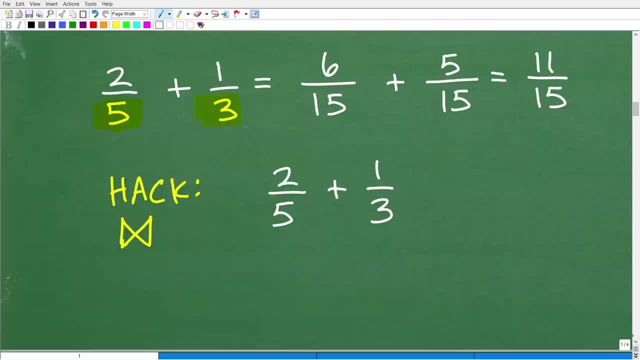 is. And you have to learn how to find the LCD. This is very, very important. However, what I'm doing in this little lesson is giving you a shortcut. All right, so if I have this fraction, two fifths plus one third, I want to add these together, but they don't have the same denominator. So I'm going to have to rewrite this fraction and this fraction such that they do have the same denominator. Okay, so I'm going to have to write two fifths as I'm going to have to find an equivalent fraction of two fifths. 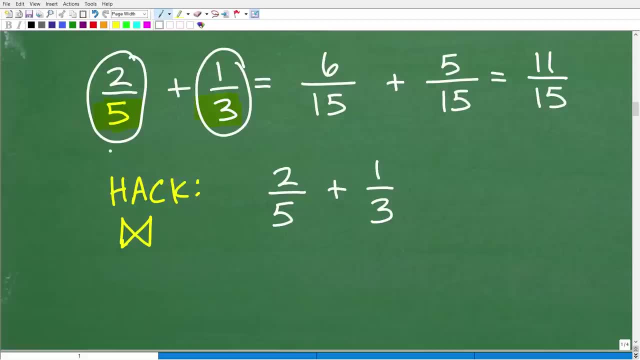 Okay, it's the same thing as two fifths, but it has a denominator is going to be the same as an equivalent fraction here that has the same denominator. In other words, I got to match up these denominators. And we're trying to find that same denominator that these two fractions have in common. That is the lowest common denominator. Okay. So if I most people would say, Okay, here, what is the LCD? Most of you would say it's 15. Okay, we'll probably know that. And you would be correct. Now I have additional videos on how to find LCD, it's important that you understand that. But for this particular video, let's just assume that you know that, okay, yeah, this is the lowest common denominator is 15. So that means I want to rewrite each fraction such that the denominator is 15. Okay, so here, how do I turn this five into 15? What I have to multiply it by three. Okay. So if I multiply the denominator by three, I also have to multiply the numerator by three. And that's how I get three times two, this is six over 15. So that's how this first fraction right here, I rewrite as six over 15. And then a one third, how do I get this to be a 15, I multiply by five, so I'm going to multiply the numerator by five. So I get five over 15. So I'm showing you kind of the long way that we deal with fractions. Okay, this is probably the way most of you have learned this problem, or learn how to add or subtract fractions. And that's perfectly fine. Again, I'm going to show you a nice little shortcut here in a second. But now I rewrote 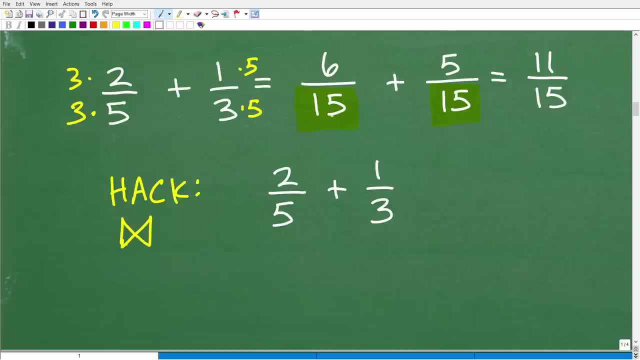 these fractions such that they have the common denominator, the lowest common denominator. So remember the rule, when the denominators are the same, I simply go ahead and add or subtract the respective numerators. So this is six plus five, of course, that's 11. So I got 11 15. Okay, so that is the answer. And this is the way most of you have learned this using the LCD method. Okay, so we'll go ahead and put this here LCD. But hey, what 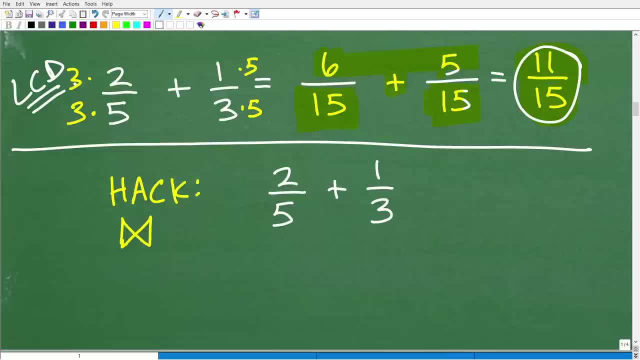 if you don't want to deal with LCD? Well, you're in luck, because you're watching this video, I want you to remember this little symbol right here. Okay, it's called a bow tie. Okay, just like you wear a little bow tie. I don't think too many people wear bow ties anymore. But this is the general pattern I want you to remember. Okay, this is going to be super, super easy. This works with variables, it works with any addition or subtraction, fraction problem, you will get the answer right 100% of the time. Okay, so here we go. I want to show you how easy this is. Here's the pattern. You start in the bottom right and you go this way. 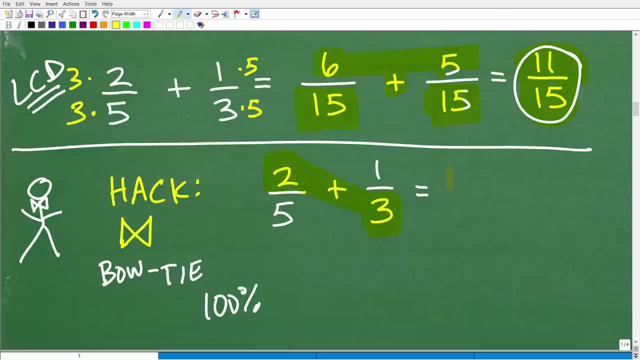 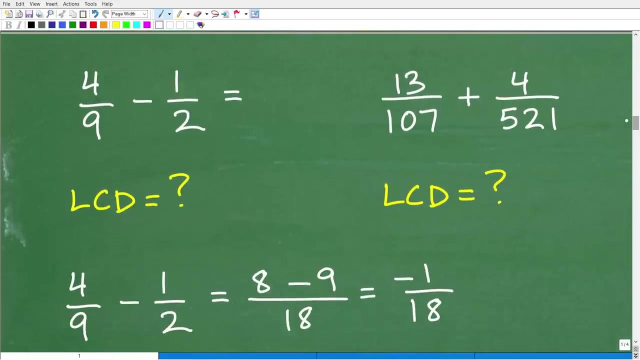 Okay, you always start from the bottom right. And you go this way first. Okay, so we're going to do three times two, we're going to put our answer there. And then you're going to go from the bottom left and go and go this way. So you can see it has like a little crisscross pattern. We're going to put that answer there. So let's do that now three times two is what six. Now this is an addition problem that's going to be plus five times one is what five. Okay, that's our numerator. So this times this always start from here. Okay, because this, this will make an impact if you're subtracting fractions. So three times two is six, plus five times one is five over our denominator is going to be five times three. So here's our bow tie. Five times three is 15. Now we simplify that six plus five it is exactly the same thing we have right here. But look, I didn't have to mess around and change these fractions even think about the LCD. I simply just thought about a little about my little bow tie method. I went this times this, plus this times this over this times this. Okay, this is the bow tie method, you're going to want to know this, not only for arithmetic, but for variable fractions as well. So let's go ahead and practice this right now. Okay, so okay, so 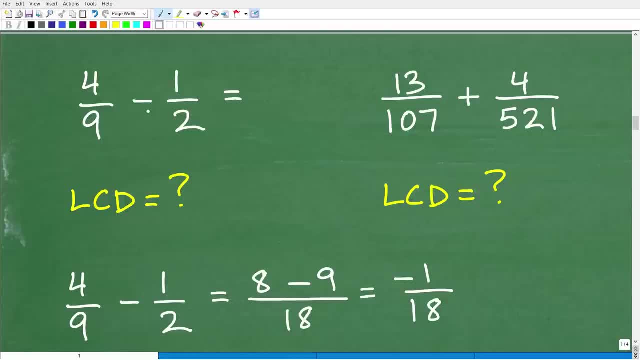 So let's take a look at this problem here. Four nights minus one half. OK, so what is the LCD of this problem right here? OK, well, everyone, you know, we're looking at this video right now. You can see I kind of wrote it, but most of you hopefully could say, well, the LCD is 18. So that's good. If you know that the LCD is 18, that's excellent. 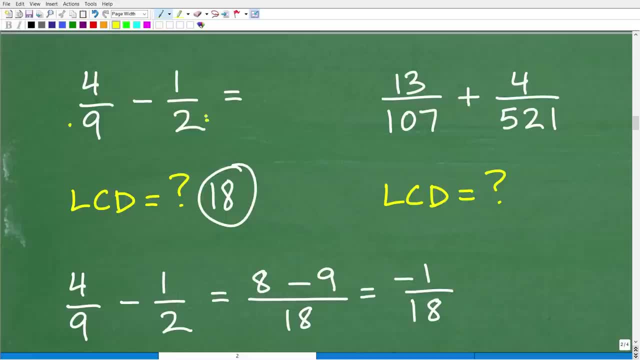 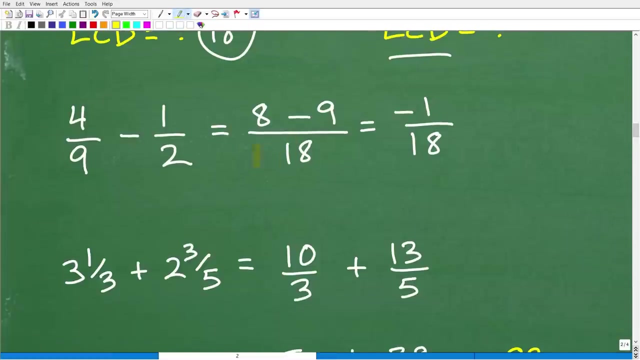 So you can, you know, write each of these denominators as 18. You're like, well, I would just multiply this by two and this by nine. And now I'm going to go ahead and fix this thing up right here and, you know, use the LCD method. So some of you may be nonbelievers in the LCD, this little bowtie method. I'm actually saying you're like, no, I'll just stick with LCD. And that's good. You need to know that. But what about this situation? OK, what's the LCD between these two denominators? OK, now this is where it gets fun because most people are going to be like, all right, I'm not watching your video anymore. I'm not doing this problem. OK, so to find the LCD of these two denominators, this gets much more interesting. All right. So a lot of you are like, oh, OK, OK, I'll maybe I'll just use your bowtie method because to do this problem, it's super easy. I would just go this times this plus this times this over this times this. Now I'm going to have big numbers, but I will add these fractions. And I will have the exact right answer. The only thing with the bowtie method is that oftentimes, well, not oftentimes, sometimes you're going to need to reduce your final answer, but your answer will be correct. But you may need to reduce your final answer, but you will have an accurate answer. OK, so that's the main idea. All right. So let's go ahead and practice this bowtie method right now. OK, so again, let's take a look at this first problem. We're not going to be thinking about the LCD. We're going to go, OK, I'm going to start from the bottom right. I'm going to multiply this way. OK, so two times four, that's eight. This is a subtraction problem. So I have a subtraction operator there. And then nine times one is nine. And then my denominator is going to be nine times two, which, of course, is 18. 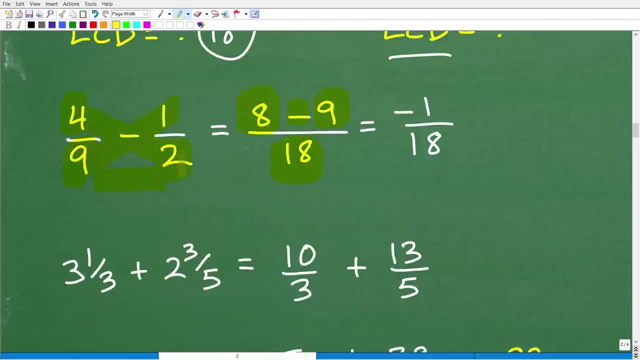 Now, when you're subtracting fractions, especially, that's why the order is very, very important. That's why you have to start. 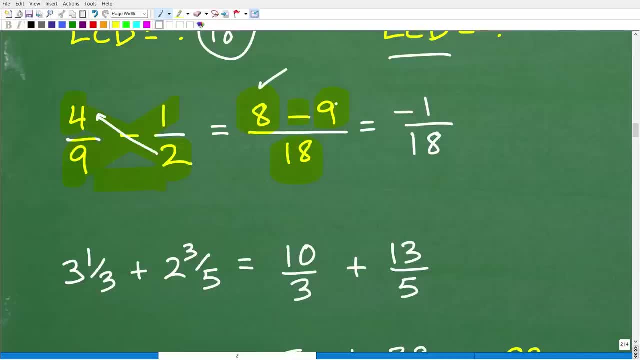 This way, OK, because we have our eight there. If you put your eight right here, you would have a different sign. So when you're subtracting fractions or subtracting any number, you've got to be very, very careful that you have the correct sign. 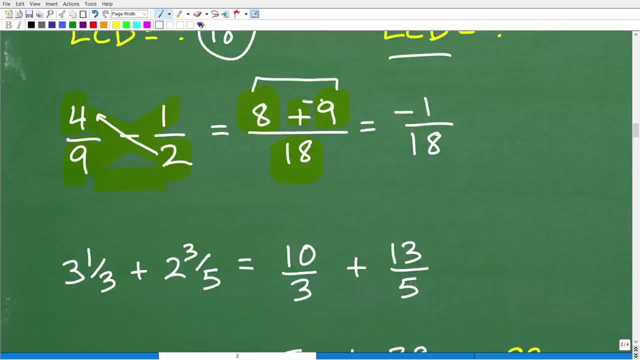 So eight minus nine is the same thing as eight plus a negative nine, which is negative one. OK, so the final answer here is negative one over 18. OK, negative one over 18. That is the answer. But again, we're using that bowtie method. All right. 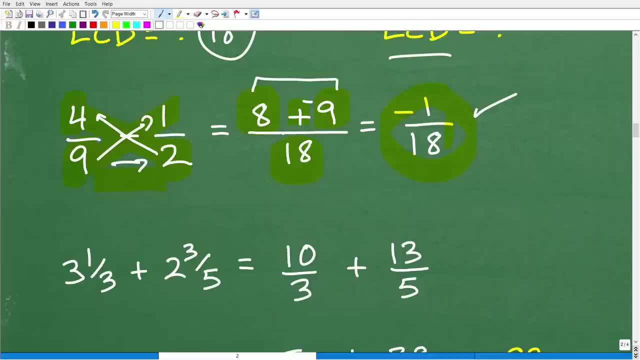 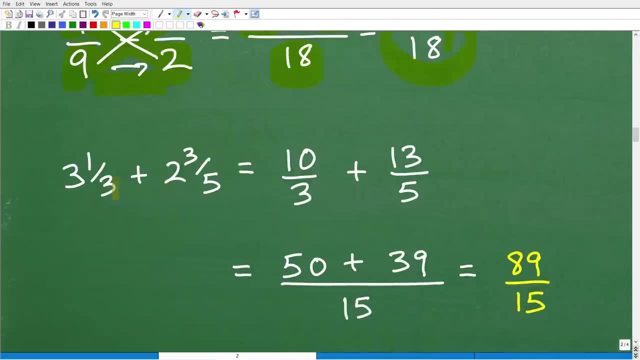 When I have to think about it, I just have to follow the procedure and make sure I do the arithmetic correctly. All right. So how does this work with mixed number fractions? So basically the same way we did with multiplication division, we want to rewrite each of these respective mixed number fractions as improper fractions. 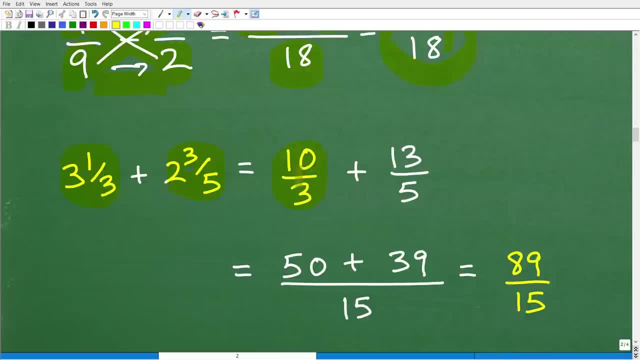 So three and one third is the same thing as ten thirds. And then two and three fifths is the same thing as thirteen fifths. So now I can go ahead and just do the bowtie method. So that's five times. 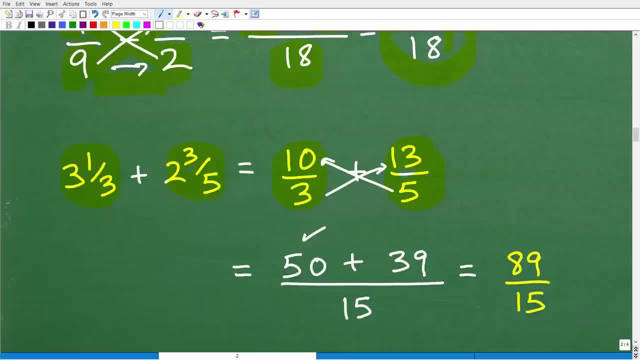 Ten is fifty. Three times thirteen is thirty nine over three times five, which is fifteen. And I'm just going to go ahead and add my numerators. Fifty plus thirty nine. That's eighty nine over fifteen. And we are done. OK, so hopefully your facial expression about fractions went from here or maybe like it was total confusion from here to here to here to a big, lovely, happy face. OK, this is the whole idea behind this. OK.